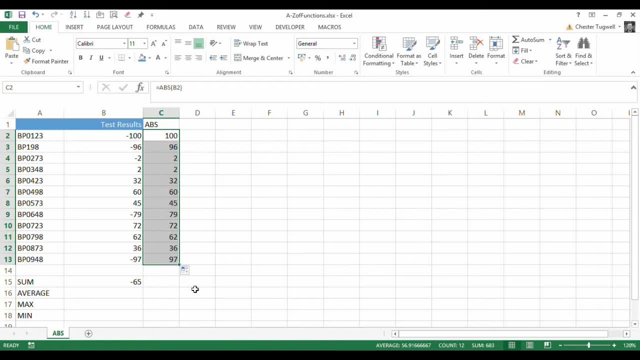 version of that number, which is the number without its sign, and then what I could do is just add those up. However, that's the answer I want, but really I want it there. I don't want to really have a second column with another version of the numbers. I want to do the whole thing in this cell here. Now, that is possible. 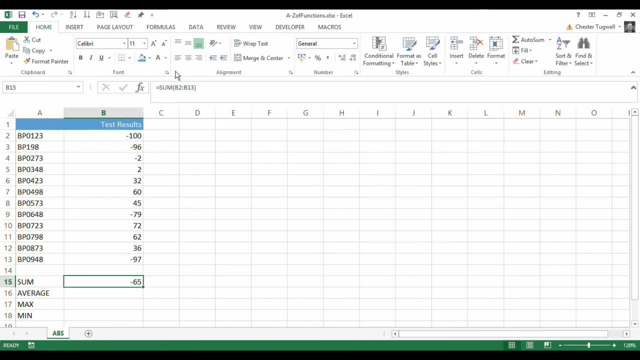 Let's just take that out Now. what I need to do is sum up the absolute version of this range, The absolute version of this range here. Now let's just see if we can do that. So what I'm doing is I'm saying, instead of summing up b2 to b13 as it is, 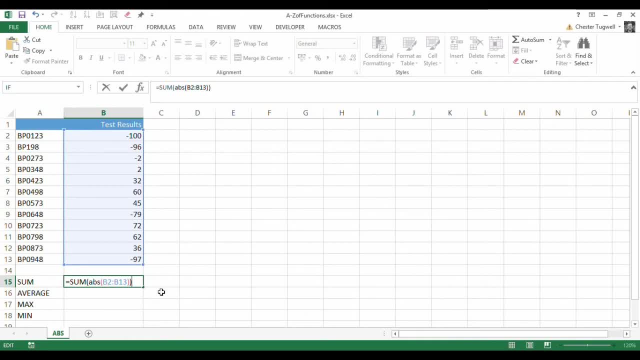 convert it to its absolute version and then add it up. Press enter. Oh dear, I get a hash value error, So it's not working. That's because abs is expecting to work on a single value rather than a range. Now what you can do to get around this is to convert this formula to an array formula. 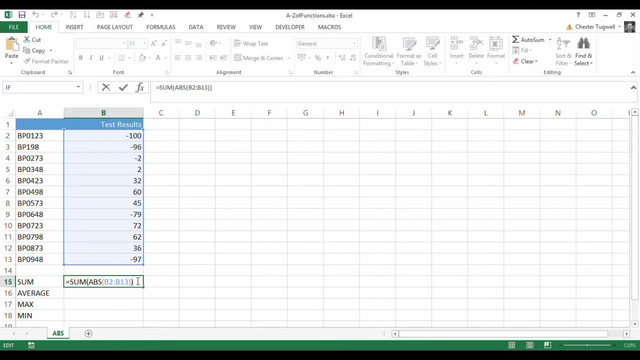 Now, normally when we press, when we want to confirm a function, we press enter. but instead, if you press ctrl, shift, enter, you create what's called an array formula. Now you can see the effect of that is put these brace brackets on either side of the formula. That tells me that I've created an array formula. 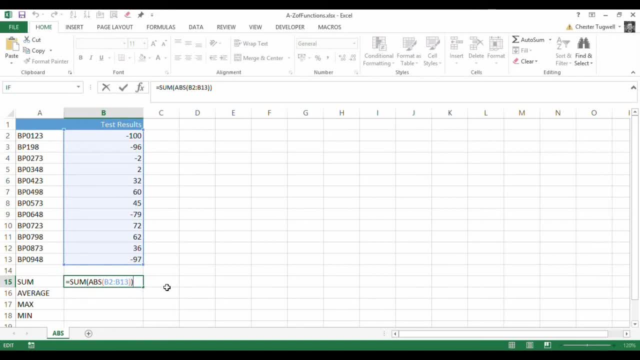 So the trick was just to go back: instead of pressing enter, I press ctrl shift and enter, and that has added up the absolute versions of those numbers. I could do the same with average, So I'm selecting the results. Two close brackets, ctrl shift, enter. Now I've got the average. 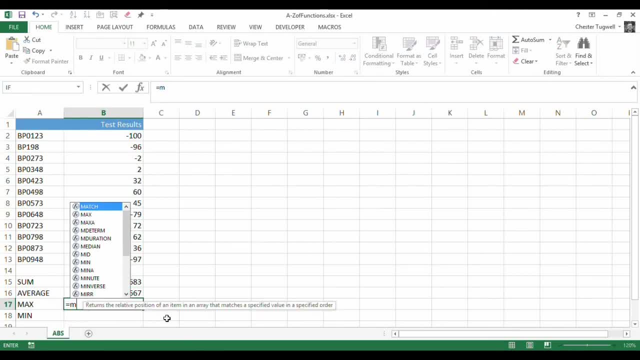 The minimum. now that's quite interesting. So if I say equals, sorry, the max, Same same idea. Select the range, Two close brackets, ctrl shift and enter, So it's returned 100, even though the 100 is actually the negative figure or the smallest figure.